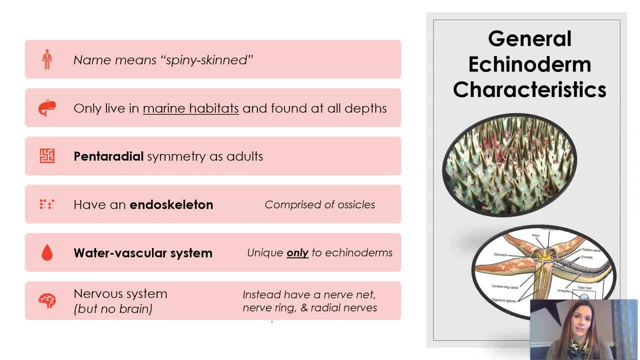 things arranged in fives. They also have an endoskeleton. So up until now we've really been focusing on exoskeleton organisms. but echinoderms have an endoskeleton and it's comprised of ossicles. They also have something called a water vascular system. that is unique to only the echinoderms. So we're going to start with the echinoderms and we're going to start with the echinoderms. So we're going to start with the echinoderms and we're going to start with the. 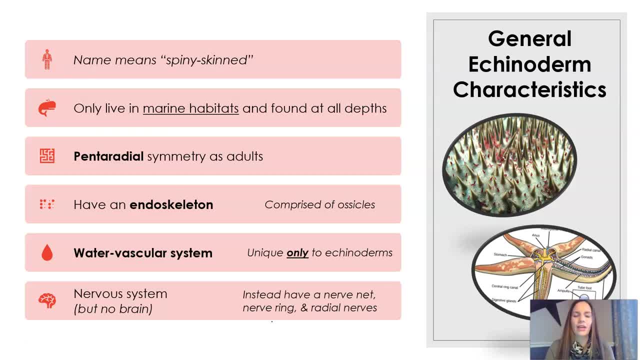 They are the only organisms that have this system- and when we get into it in a minute it's pretty cool too- And they also have a nervous system, but no brain. So we still don't have a well-developed brain, but there is still a nerve net and some other nerves going on within the body. 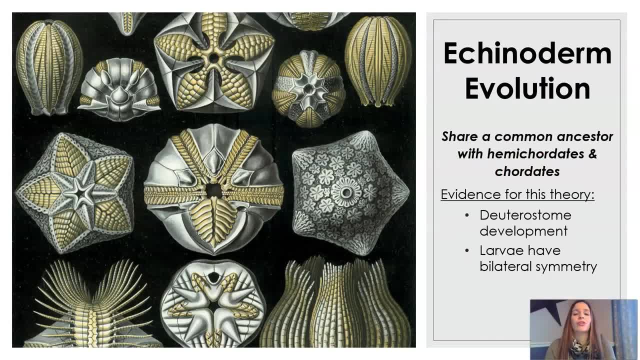 A little bit about the evolution before we get into some of the diversity of the phylum. So echinoderms are being discussed at this point in the semester because they share a common ancestor with hemichordates and chordates Like us. That being said, there's a little bit of evidence for that. First of all, they have 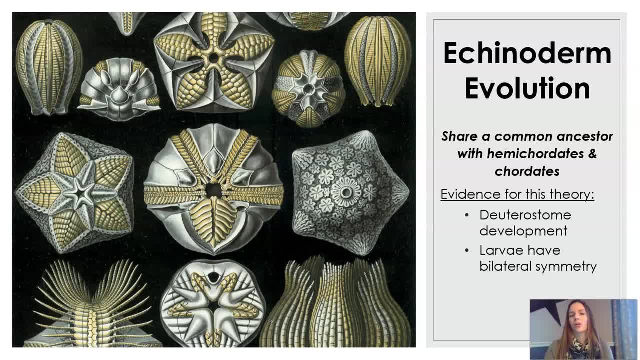 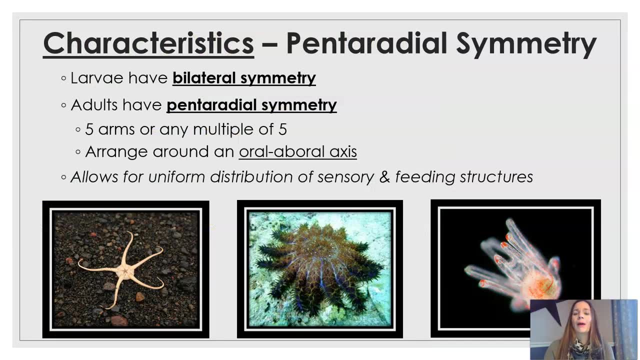 deuterostome development. So up until now we've been discussing organisms with protostome development. These are the first ones with deuterostome. They also have bilateral symmetry as a larval form, showing that there is some sort of common ancestor there. So a little bit more. 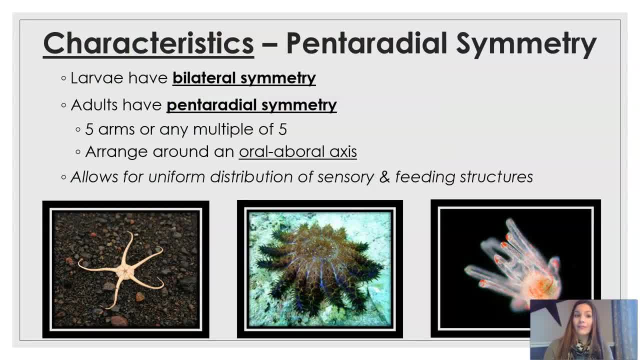 about pentaradial symmetry. So penta is five. So the larvae have the bilateral symmetry, but once they develop into adults they have this pentaradial symmetry in fives. So when we think of an echinoderm or a starfish or a sea star, we typically think of something with five arms. 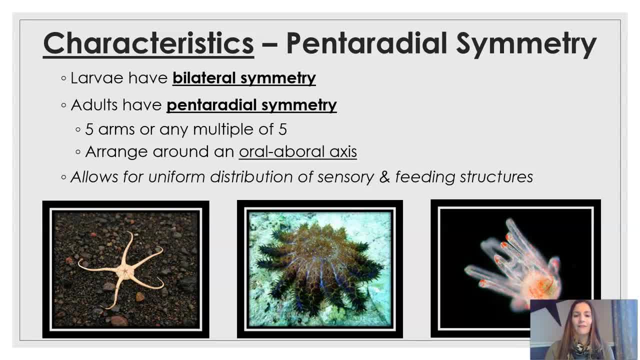 But there are others that can have multiples of five. So if you look at this organism here on the bottom in the middle, you will see there are more than five arms there, I think. actually I believe there's 15.. That's a crown of thorns, sea star, But it's also this arrangement around. 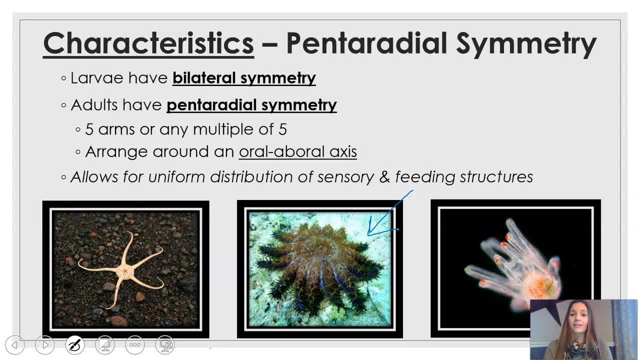 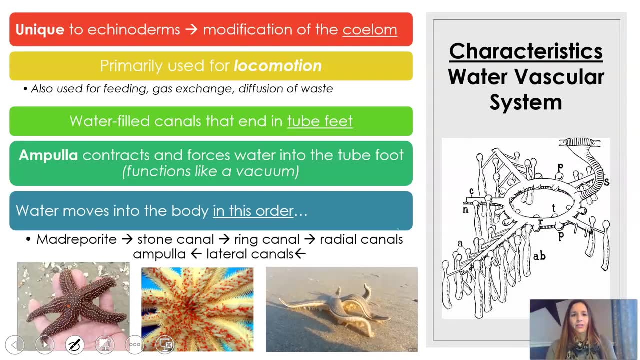 an oral-aboral axis, So the oral end is on the bottom or the mouth, and then the aboral is on the top, And this also allows for that uniform distribution. So every arm has sensory and feeding structures within it. A little bit more, then, about that water vascular system. So if you 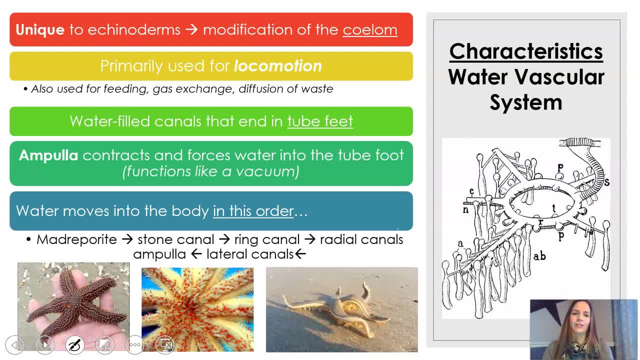 remember I said it's unique to echinoderms- They are the only organisms that have this- and it's thought to be a modification of the coelom. So remember, the coelom is that body cavity. It's for locomotion, which if you look down here in this video, you will see that, But it's. 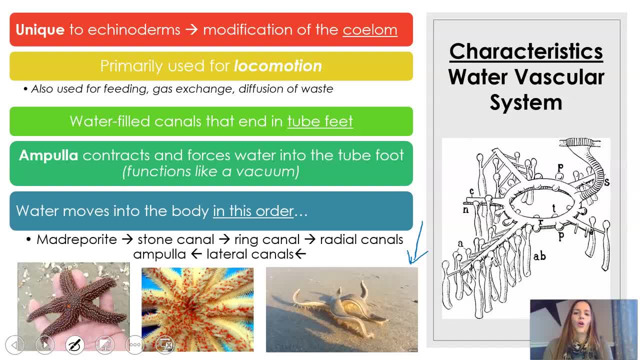 used for other things, like feeding, especially sea stars. They use it to pry open things like clams, And then it's also for gas exchange and diffusion of waste. So what it is is these water-filled canals that end in tube feet, And I think everyone's probably at some point looked at. 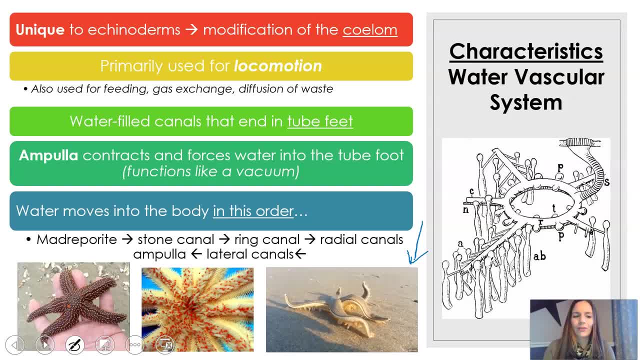 the underside of a starfish or seen pictures of one, to where you know what these tube feet are. But what happens within the sea star is that it's a tube feet And it's a tube feet that's going to contract and force water into the tube feet, which are all of these structures you see. 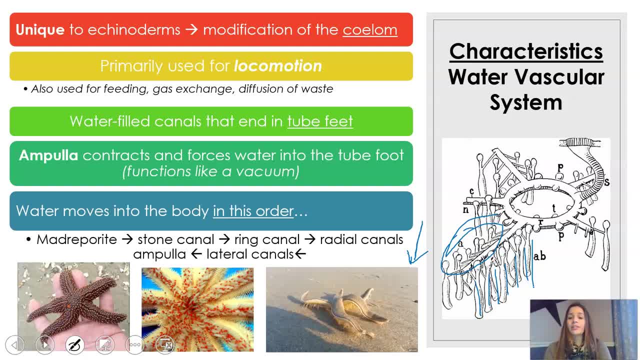 pointing down. So it's going to function almost like a vacuum to suction to the surface. That way they can move And there's a certain order that water is going to move into the sea, star or other echinoderm And it first starts with something called the echinoderm And it's going 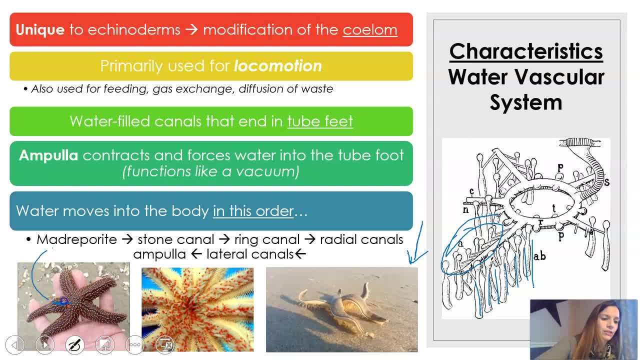 to move into the sea star or other echinoderm And it first starts with something called the magriparite. So this structure to show you is this bright orange structure you see there And it's usually pretty obvious on most sea stars when you look, because it's a different color. 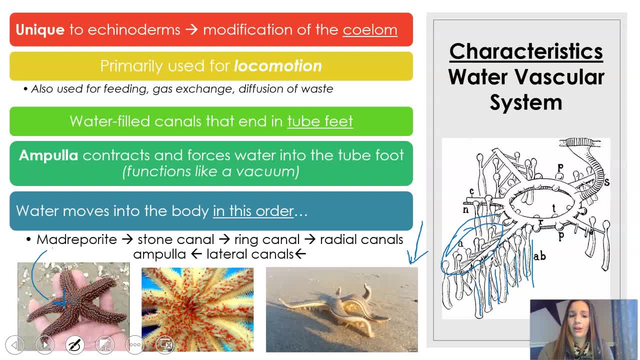 So that's where water enters. From there it's going to go into a stone canal, which is here. Then you go into your ring canal, Then you're going to go into your radial canals, which run on each arm. From there there's going to be lateral canals. So this area here is going to be. 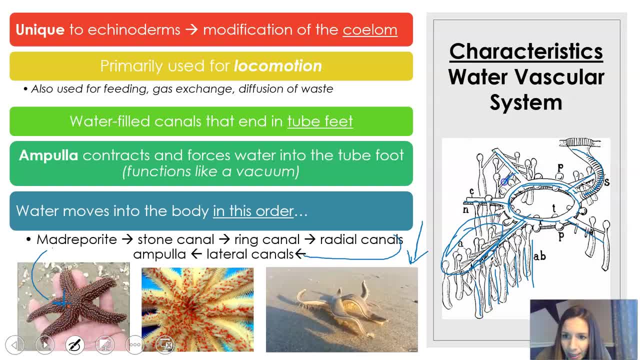 around to there. The lateral canals are these little guys you see that are feeding out to the ampulla And then from there you go to ampulla And then ultimately out the tube foot. So now that we've learned a little bit about what they can do and what they're capable of. 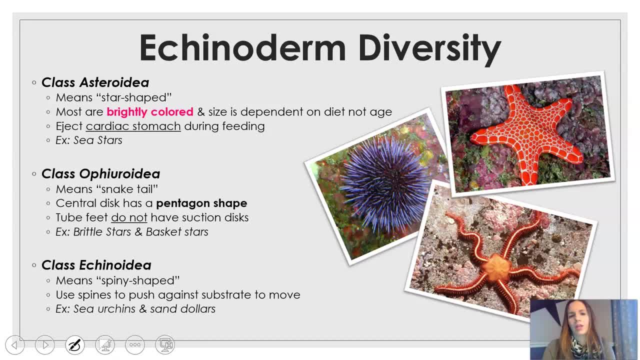 let's talk about their diversity. So the first one, and this is probably the most common one that you're familiar with, is members of class Asteroidea, And these simply mean star shape. They are usually very brightly colored, But, interestingly enough, 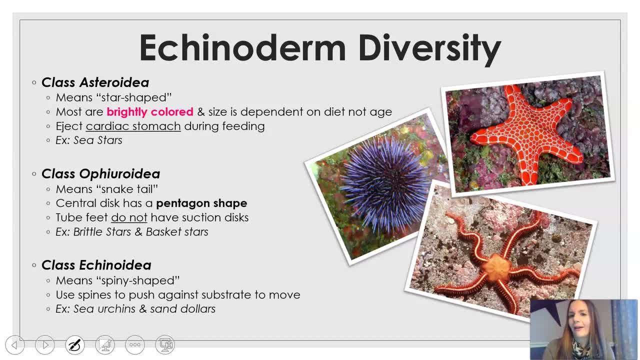 size as they grow is not dependent on how old they are. It's dependent on how much they eat. So sea stars in areas with a large selection of food items are going to grow faster and be larger than ones that may be in a more restrictive environment. And something interesting as well. 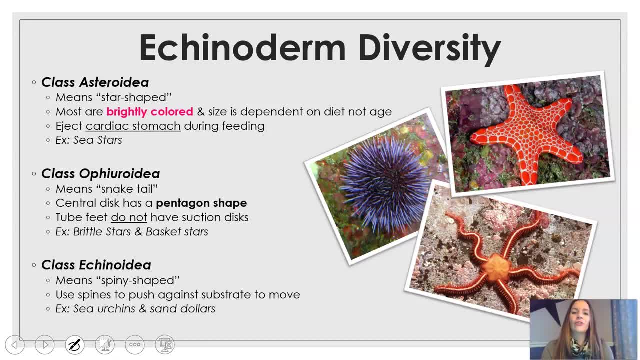 is they can actually eject their cardiac stomach when they eat, So they will eject it out and it almost starts breaking down the organism right away before they bring it in for the rest of digestion. And that example, like I said, is sea stars, which you can see in the picture, And so 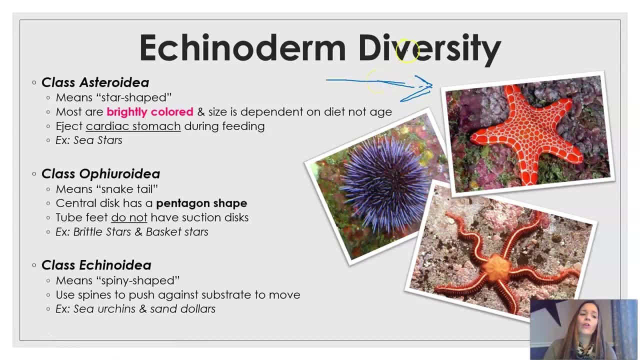 you see here. Next up is class Ophigeroidea, And these are a little bit different but they're very similar to starfish or sea stars because they do still have kind of these arms all the way around them And they do exist in fives but also in tens and other multiples of five, But their 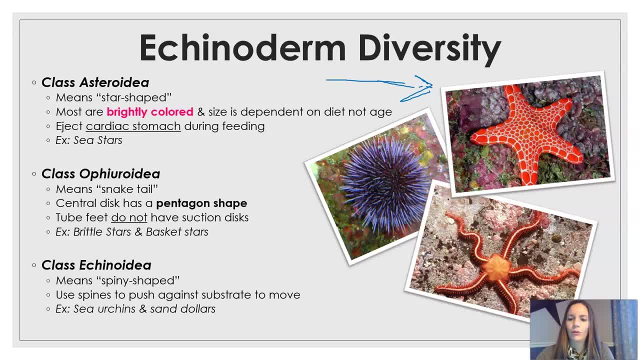 central disc is a little different because it has a pentagon shape. So if you look at this picture here, you see that pentagon shape in the middle and then you see the arms. But their tube are also a little bit different because they don't have the little suction discs like sea. 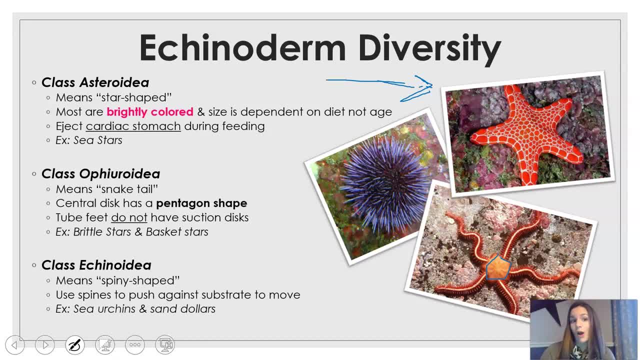 stars do So. they kind of flail around like a snake in the water, which is where their meaning comes from of snake tail. So that's this picture here, And then the last one on this slide is class Echinodia, which are spiny shaped. So we had spiny skinned as the meaning of the entire phylum. but 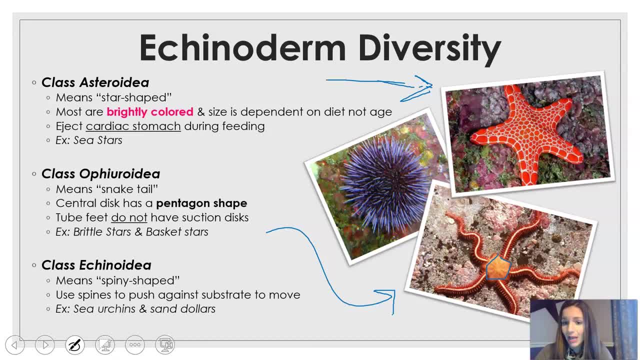 this class. it means spiny shaped and that's because they have spines, So things like sea urchins, which is here, and they actually move by pushing those spines against the sand. The last two that we're going to classes we're going to discuss within this phylum is first up. 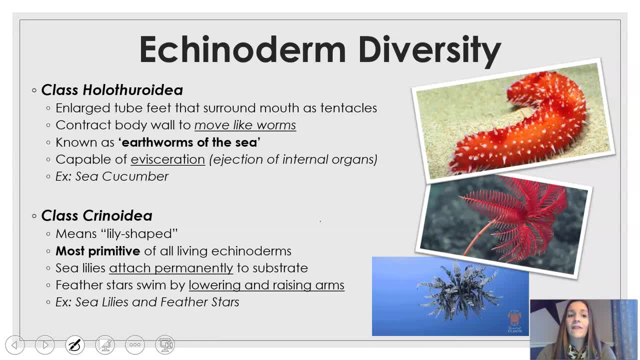 class Holothoroidea and these are sea cucumbers And these are pretty cool. So at first glance you wouldn't expect them to be related to sea stars or brittle stars. but they do have tube feet and those are actually enlarged and they go around the mouth kind of like tentacles. 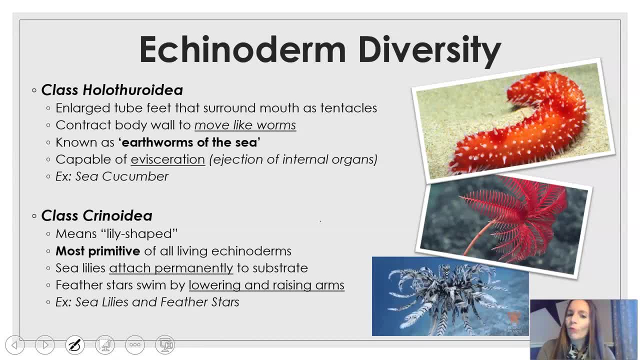 And we'll talk more about that feeding process In a minute. but they move like worms and they're actually known as the earthworms of the sea because they can. they feed on the bottom and they kind of turn over the seafloor. 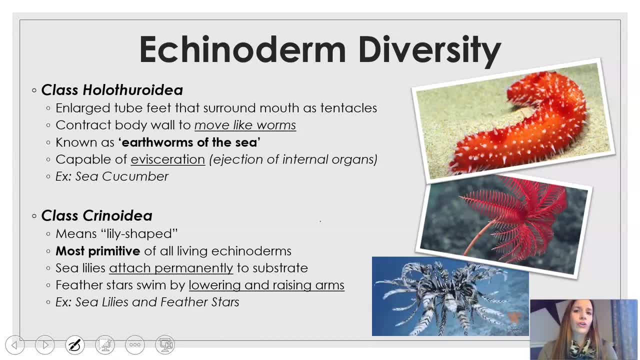 much like earthworms do on the soil: They feed on the soil, they turn it over, they're good for it. So they're earthworms of the sea, and they are capable of something pretty cool called evisceration, which means they literally eject their guts out to scare. 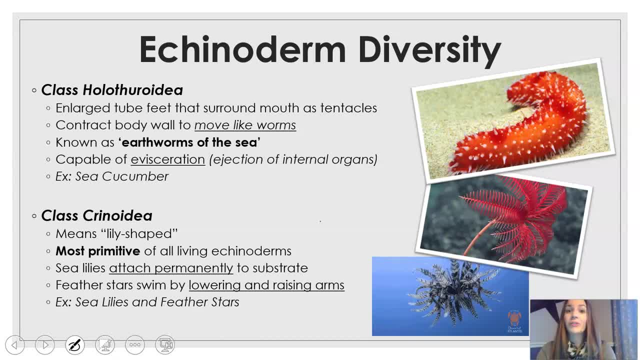 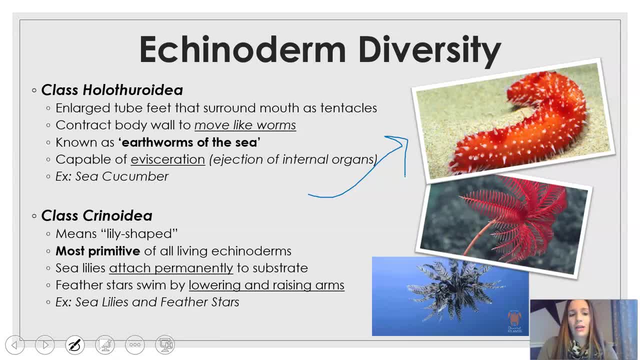 class is class chronoidia, And this name means lily shaped, And these are actually the most primitive or the oldest of oleokinoderms And they have two major types. So first there's sea lilies, which are here, and those attach permanently to the substrate where they live, And then you. 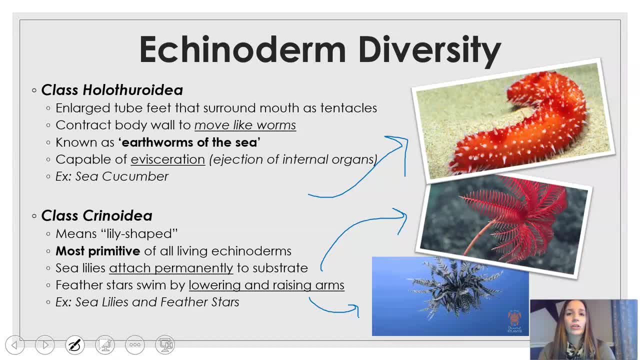 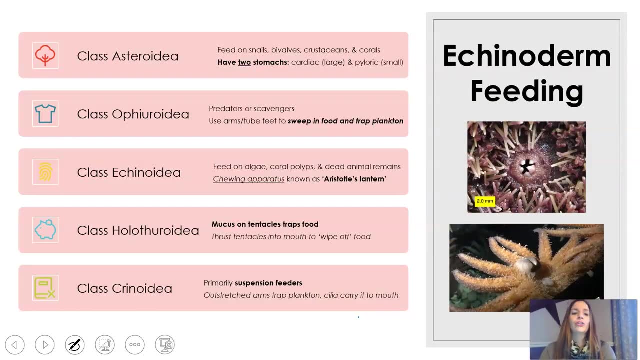 have something called feather stars, which at first glance probably looks like a pretty decent Photoshop job, But these are legitimate organisms and they look like feathers, but they are actually related to starfish or sea stars. So now that we've learned about the five major classes, we're going to talk. 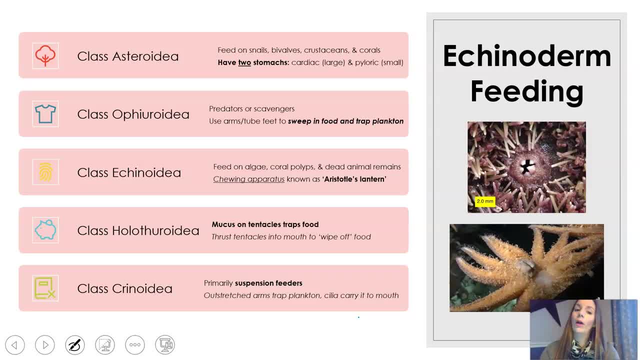 a little bit more about their feeding, because it's a little different by each one. So class asteroidia- and these are the ones that we'll probably spend the most time on in class- They have two stomachs, So that cardiac stomach, which they can eject, and then the pyloric stomach. 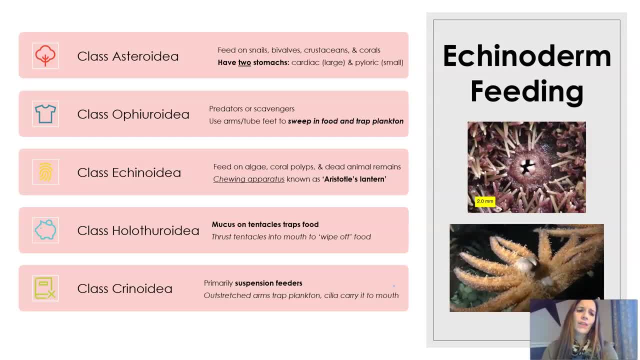 which is inside and kind of receives that broken down matter. The snake tails are the class of ophiroidias. These actually use those arms So they don't crawl like sea stars. They use those arms to sweep food into their mouth and trap plankton, Echinodia, feed on algae and coral polyps and dead animal moraines, And they 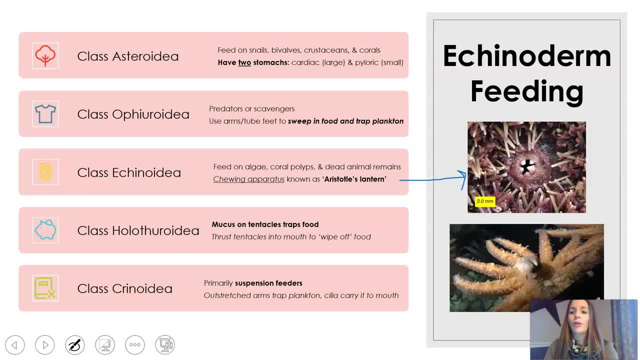 have something called Aristotle's lantern, which you can see up close in this picture over here. Oh, and I forgot to mention this- is an example of the cardiac stomach coming out. If you look at that white structure there, that's the cardiac stomach and it's actually eating a bivalve Class holothroidia. 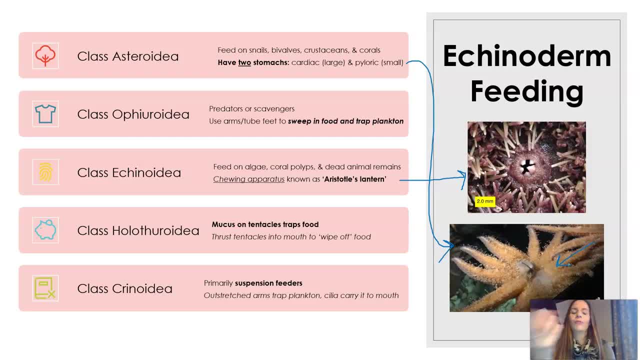 like I mentioned, they have those tentacles and they're ejecting or not ejecting, but they're getting things and bringing them into their mouth, So they're going to kind of wipe off. It's like you sucking off your fingers after you eat chicken wings or something like that- And then last up. 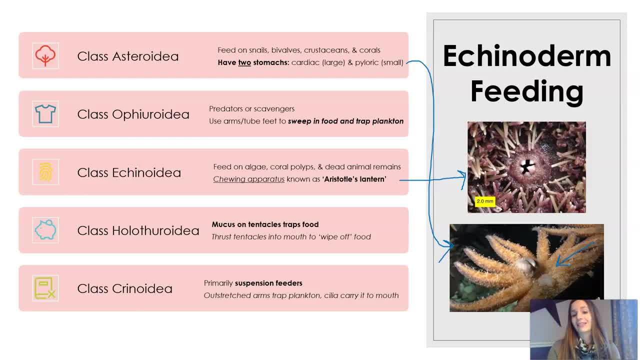 class crinoidia. these are your suspension feeders. So remember that, like sea, lilies are stationary, They can't move, So they kind of rely on things to get trapped in their arms and then it gets carried to their mouth. with cilia, In terms of reproduction, they are also. 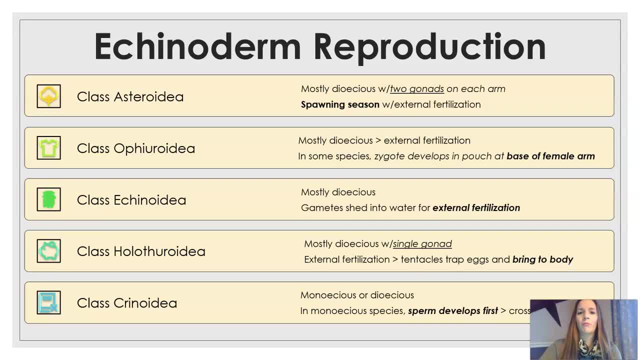 a little bit different, but for the most part. you're going to notice a term come up a lot which is dioecious. Dioecious means that they have separate organs in males and females, So class asteroidia. these are pretty cool the way they reproduce. They have these extreme spawning. 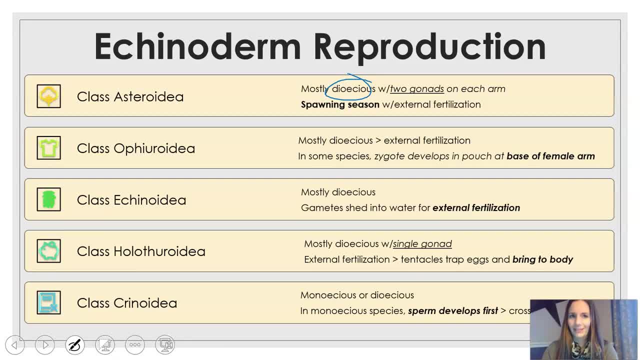 seasons and they can actually release like over 2 million eggs at a time per individual. It's crazy. Of course, external fertilization happens And during the spawning season it's dependent on things like daylight and water temperature. The other ones have a little bit varying through, So 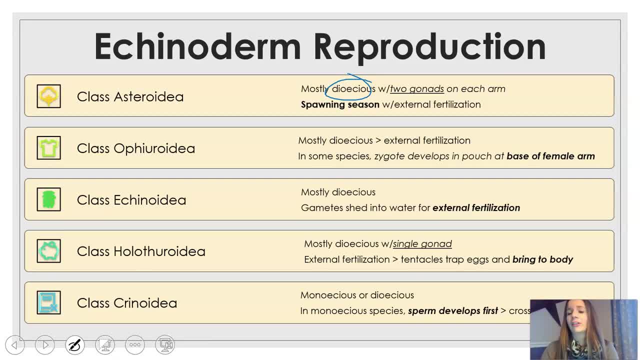 your snake tails and your brittle stars are going to also have external fertilization, but the zygote itself, so that fertilized egg is going to develop at the base of the female arm. in some species, Echinodia, do external fertilization. Sea cucumbers have a single gonad and sometimes it's kind of 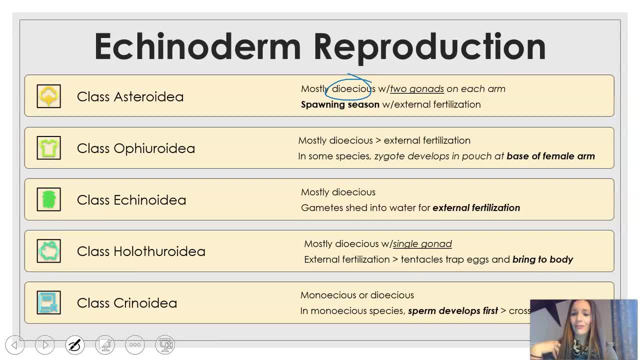 cool. They'll actually bring those fertilized eggs to their body surface and that's where they brood them or grow them as they turn into babies And then class crinoidea. they can be monoaceous or dioecious. Monoaceous meaning they have male and female organs in the same individual And in 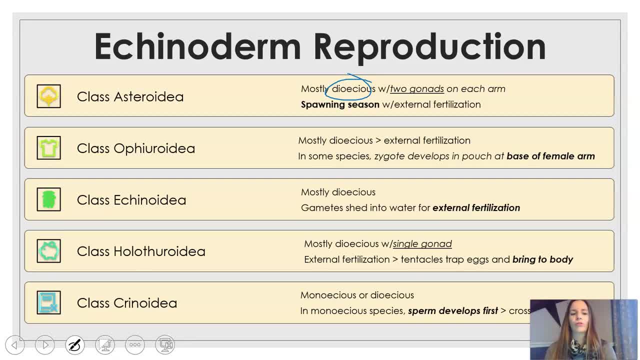 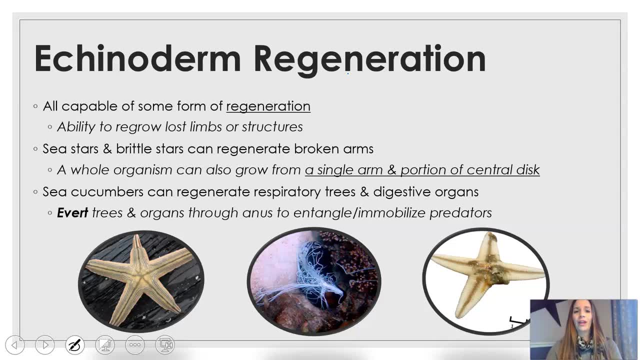 this case the sperm would develop first to still allow for some sort of cross-pollination. So something that I'm sure you're very familiar with is the fact that echinoderms are able to regenerate. So they are all capable of some form of regeneration, So they're able to regenerate. 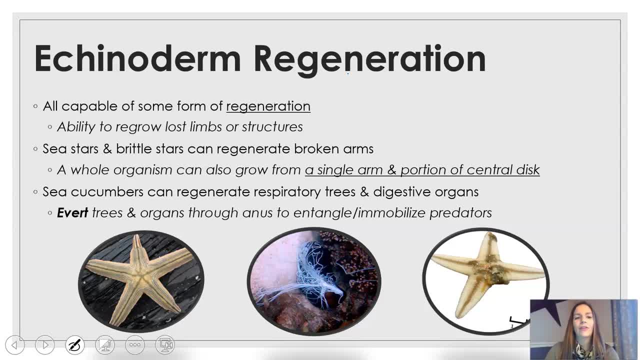 and they're able to regenerate and they're able to regenerate and they're able to regenerate. It just depends on the organism or the class and how they do it, And this is just the ability to regrow their lost limbs or structures. So sea stars and brittle stars are actually able to regenerate broken arms. 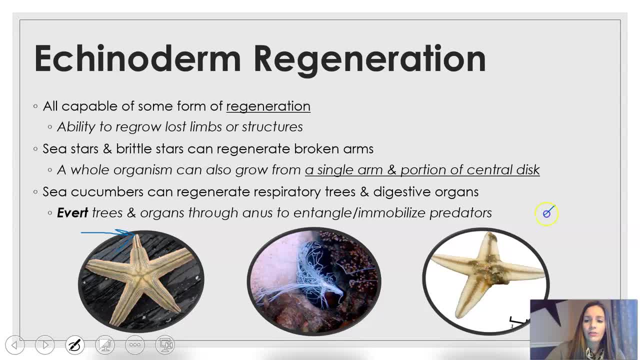 And there's two different pictures here. You see it there and you see this one here. And actually even if you just had one arm and part of that central disc or that middle section, so like if this other arm that fell off had part of the disc, that arm itself could go and 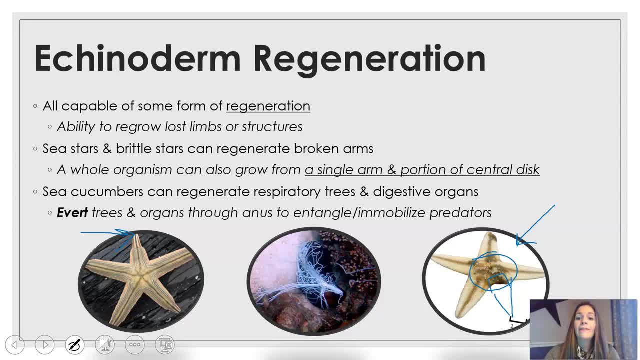 grow four more arms than the rest of the central disc. And then sea cucumbers. we talked about how they shoot out their organs and their digestive glands, but they need them again because they have to be able to continue digesting food, So they're able to regrow these organs as well. 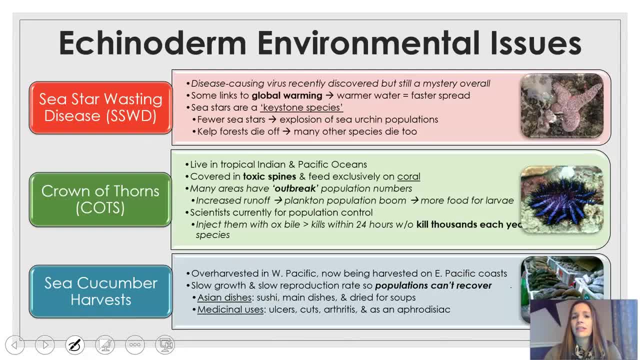 which is very important. And the last thing I want to discuss is environmental issues of echinoderms. So there's a little bit of both sides here. You have sea stars that are dying. You also have kind of invasive sea stars, And then you have sea cucumbers that are also dying in large amounts. 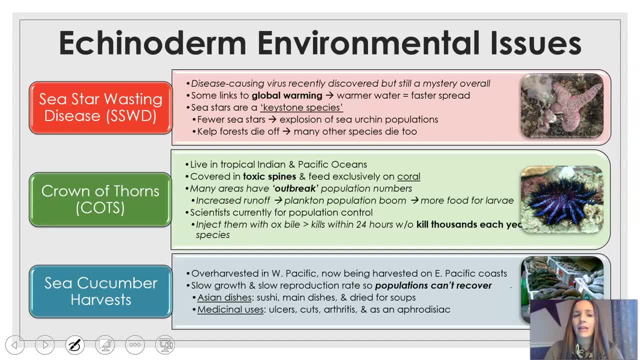 So something called sea star wasting disease has been common as of recently, and they actually just recently discovered what virus causes this disease, but it's still a mystery overall in terms of how it happens. There are links to global warming, So the warmer the ocean water becomes. 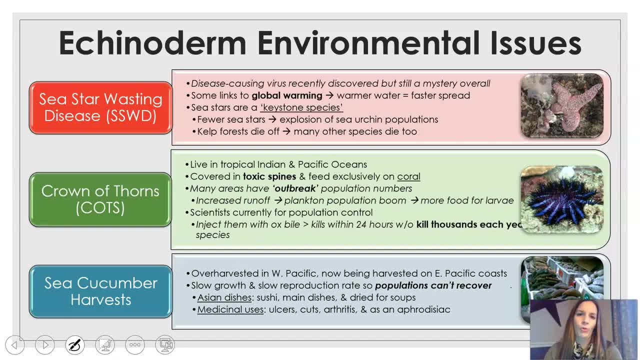 the faster this disease will spread. but it's super duper prevalent on the West coast of the United States. So California, Oregon, Washington, Canada, Alaska, they're all seeing issues with this disease And essentially the sea star like kind of wastes away. It gets kind of squishy and then it gets these splotches on it And then 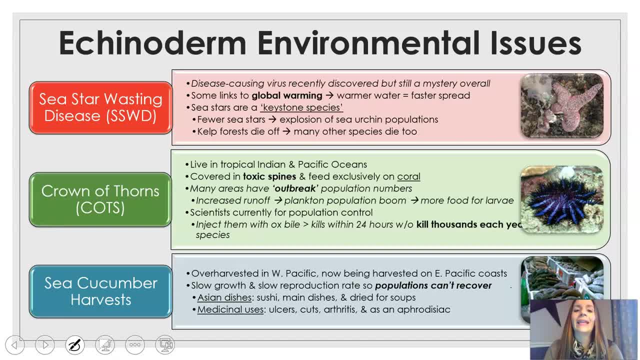 eventually it dies. Well, the problem with that is, sea stars are a keystone species, So if they're taken out of the food chain, there are so many other organisms affected, And a little breakdown of that for you is: if there's fewer sea stars, there's an explosion of sea urchin populations. 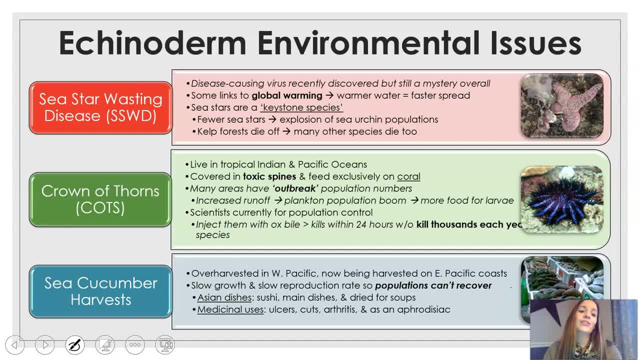 which, okay, maybe not the worst thing, right? Except sea urchins eat kelp forests, and kelp forests are home to so many other species, including those cute sea otters that we all love to watch swim around and hold hands and all that fun stuff. So 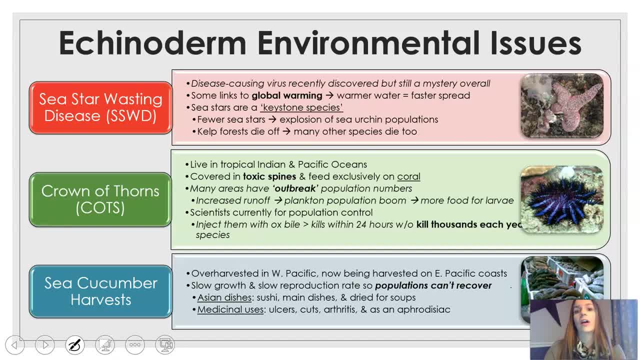 if there's less sea stars, eventually it's going to affect sea otter populations, for example. Now the crown of thorns sea star is a little bit different, because this is something that is a problem. It's causing problems. So they live in these tropical environments in the Indian Pacific. 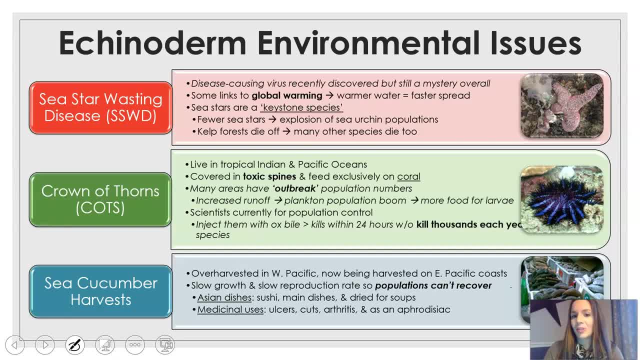 oceans. They're not in the Atlantic And they're covered with these toxic spines, which means nothing really eats them, So they don't have a natural predator and they feed on coral. Well, as you probably remember, we already have a problem. 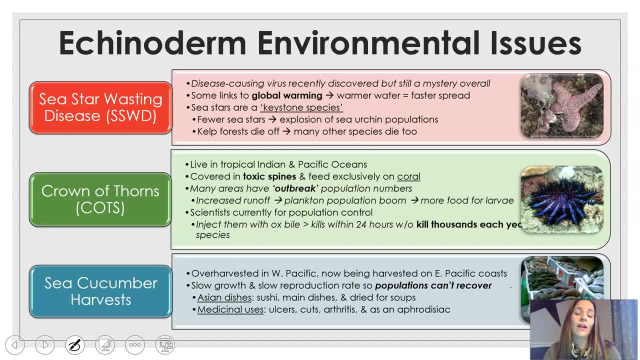 with coral bleaching and coral dying. And then you throw in outrageous numbers of these and they're eating more coral. So coral is even further affected And many areas have something called an outbreak population number, meaning they have these extreme amounts of these crown of thorns. 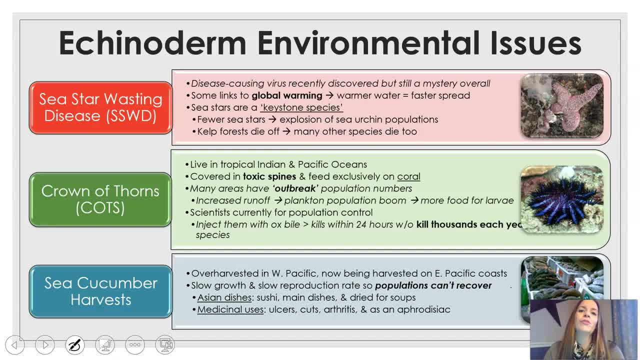 And this once again leads back to us. So we have increased runoff from farm fields and other pollution that's causing plankton to increase in population. Well, after spawning season and when you have all these crown of thorns larvae swimming around, they love that plankton, And so then you get many more that survive to become. 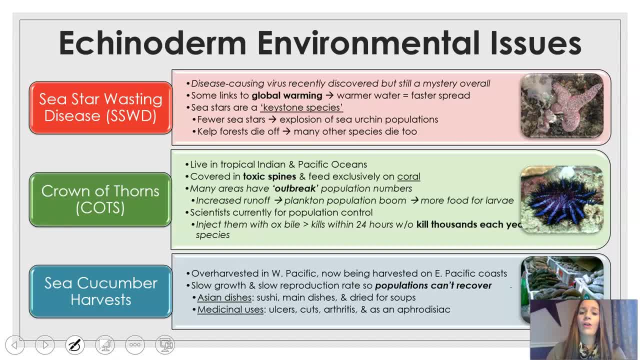 adults, And there is still population control going on right now, And they're injected with ox bile which kills them, But scientists are killing thousands each year to try to keep up with this. And, lastly, our sea cucumbers. And this is us, of course, being in the middle of the world. 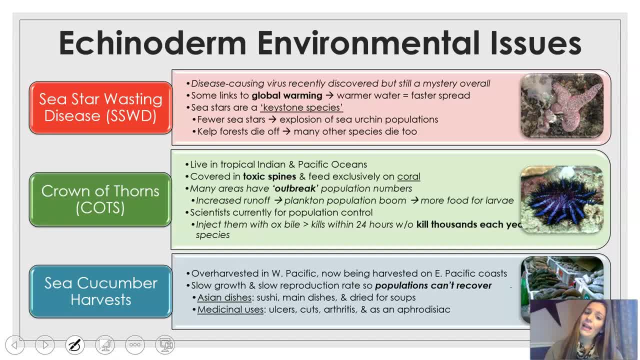 being bad again. So they were over-harvested in the Western Pacific, And now the people of Asia are coming over to the Eastern Pacific coast, aka North and South America, and harvesting them now here, because they ran out over there. Well, the problem is: 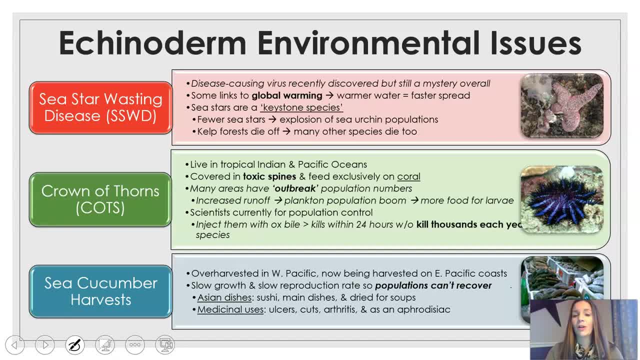 is they grow slow and they reproduce slow, So the populations can't recover, And they're very common in lots of Asian dishes and sushi, And they're also used for medicinal things. that may or may not be true, But either way we are really. 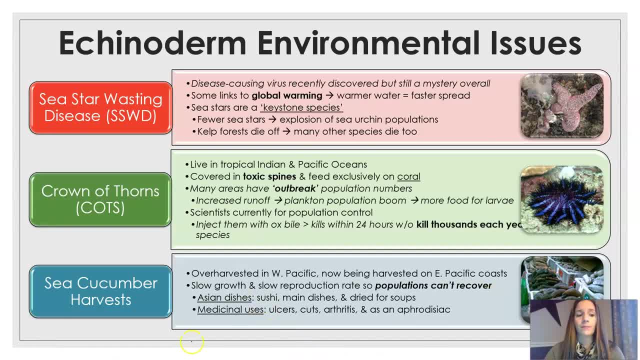 really causing some problems with sea cucumber populations. And that is all for your notes. 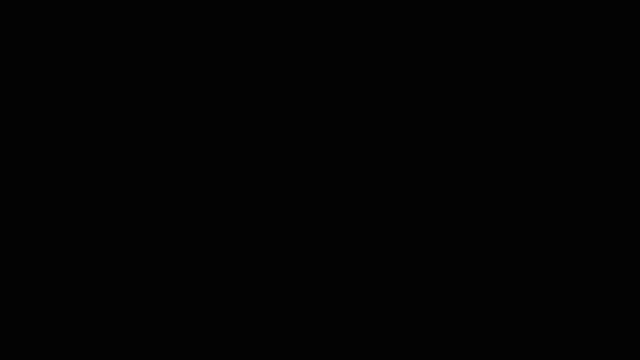 In this video we're going to talk about the formation of a cyanohydrin from a ketone. So let's begin with the overall chemical reaction. So here we have a ketone, specifically acetone, and we're going to react it with HCN- hydrogen cyanide.